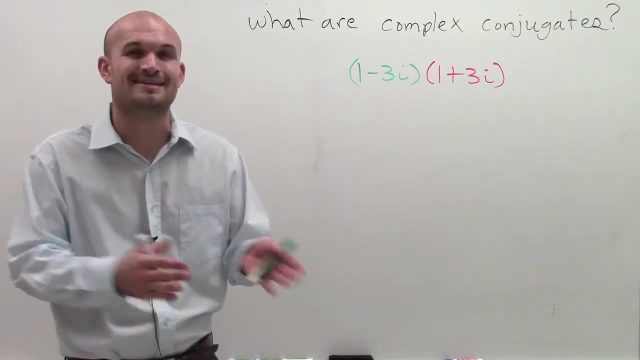 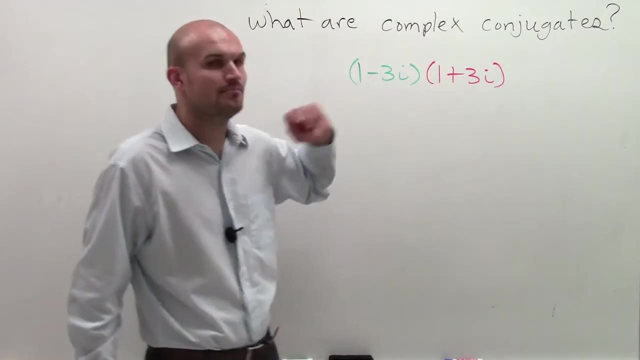 right now about complex conjugates, Because, remember, when you take a number and it's conjugate, when you multiply them, something very, very, very important happens. First off, if we look at this and we're going to multiply these, I need to notice something. 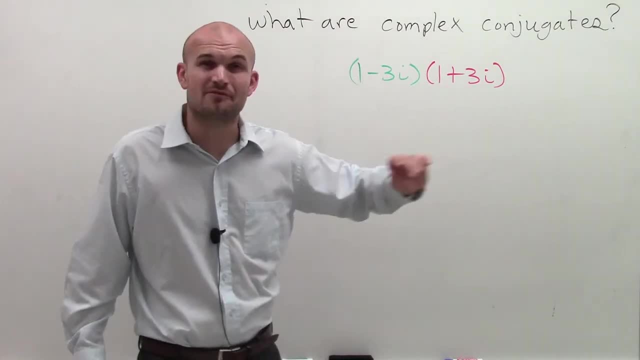 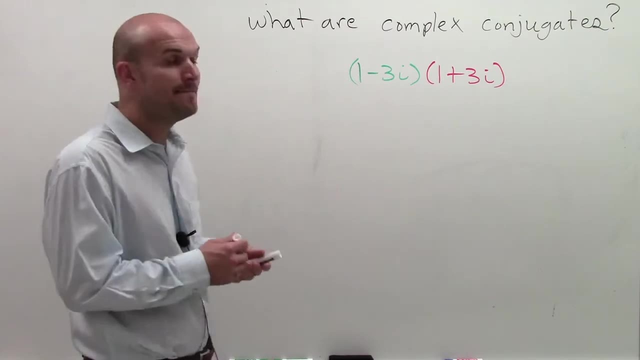 about factoring and something I've worked on, I notice that this is a difference of two squares. My first two terms are the same. my last two terms are the same, with a difference of signs, So when I multiply them out, I'm not going to multiply them out because I'm 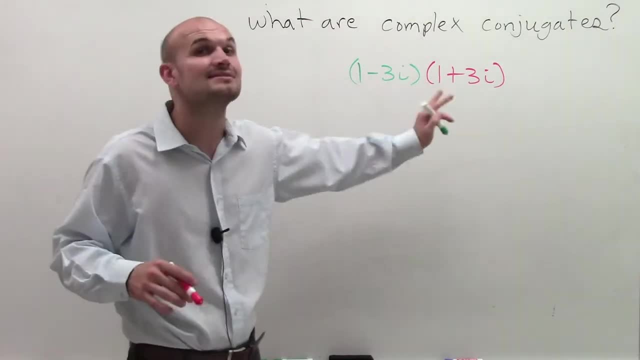 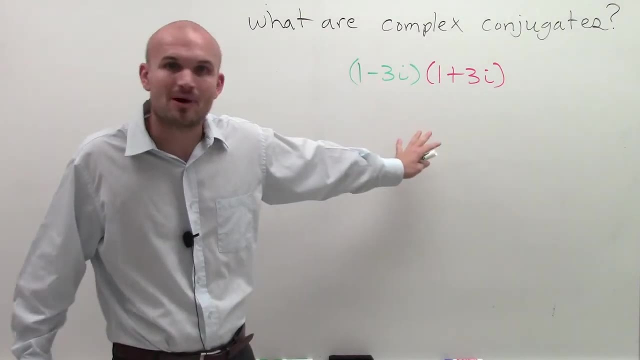 not going to waste my time nor your time. You need to understand this is a difference of two squares. When you have a difference of two squares, your middle terms are going to cancel out. Do the FOIL, whatever kind of process you want to. that's fine, but what? 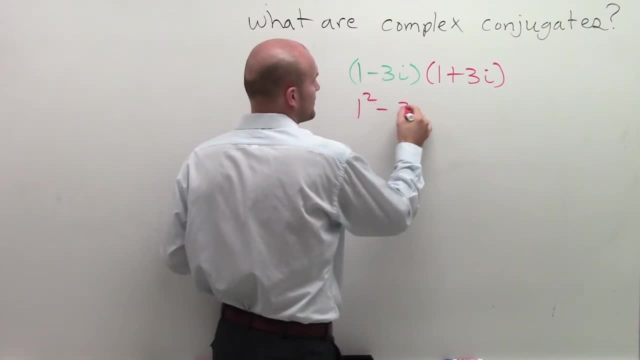 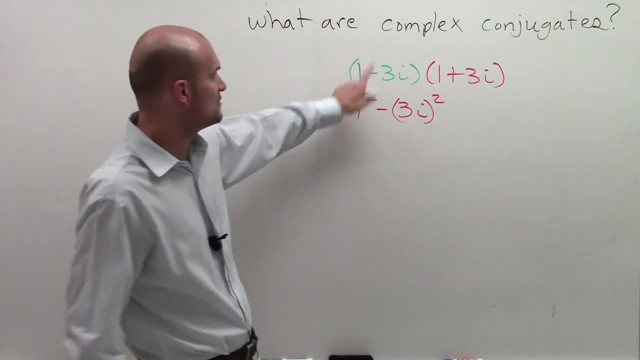 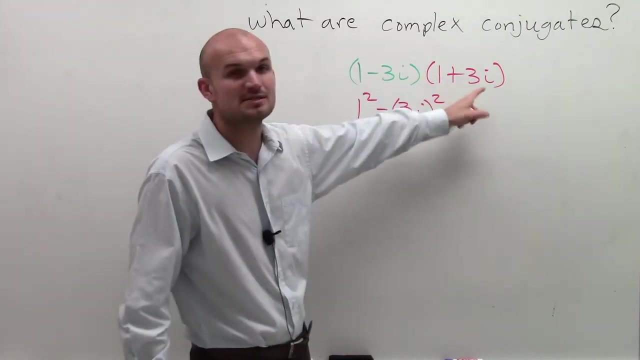 you'll notice, is you'll get one squared minus three. i squared, Alright. you multiply the first two terms and you multiply the last two terms. Now here's what's important. it's a negative because negative three times positive three is a negative. Now here's what's really cool, though, about complex numbers. So one squared. 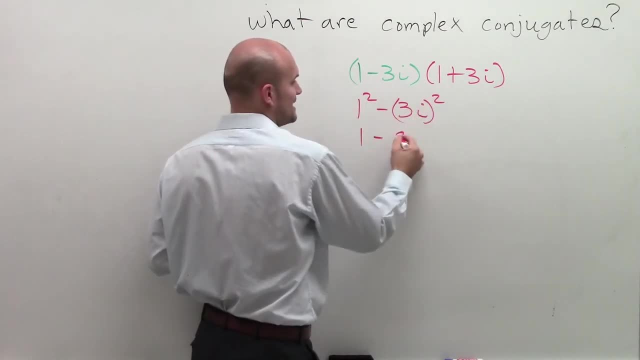 we know is one minus three squared. i squared is going to be nine: i squared. So now what we need to look at is the i number system and determine what is i squared. Well, if we said i is square root of negative one, then if i squared is one or less than i squared, then i squared is one. That's what we're looking for in this equation. That's why we're trying to determine what i squared is. Why would we say that the i squared number system is the square root of a negative one, right? Well, if we said i is the square root of a negative one, then if i squared is the, So we're. 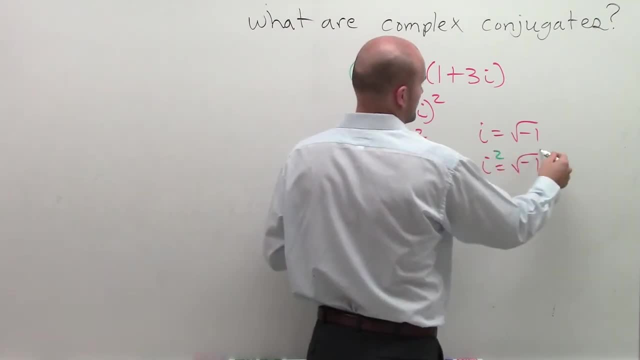 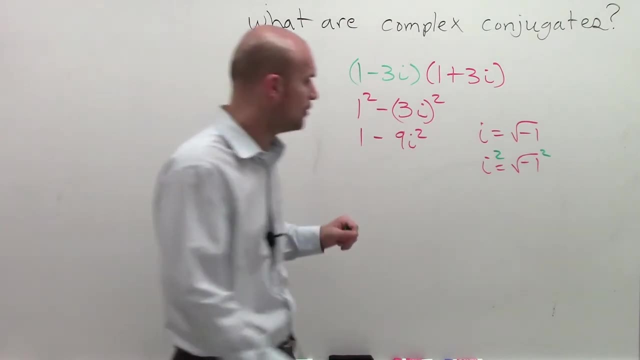 square both sides. so if I introduce the squaring of both sides, which is the squaring property of equality, as long as I do it on both sides, I'm cool, I will get. i squared equals the square root. squared just leaves me with negative 1.. 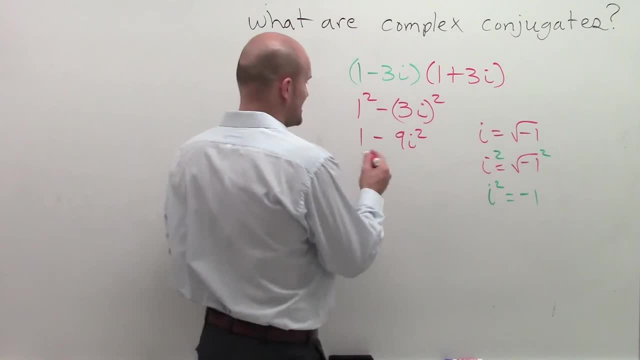 So that means now, i can now be written. i squared, I'm sorry- can now be rewritten as negative 1.. Well, negative 9 times negative 1 is a positive 9.. So my final solution is 10.. So what happens when I take a complex number? 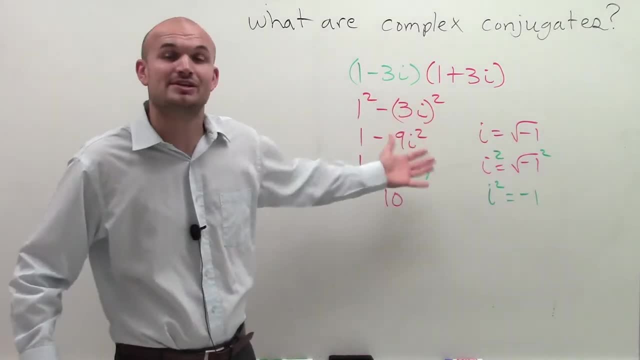 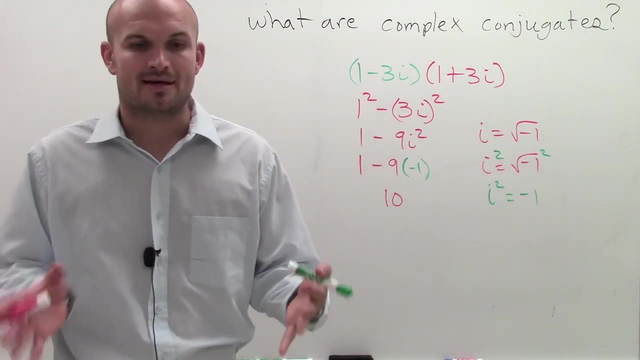 and I multiply it by its conjugate, I get rid of my imaginary number system. I don't have a complex number or an imaginary number, And that's why it's so important. So if you have a complex number and you need to get rid of it,